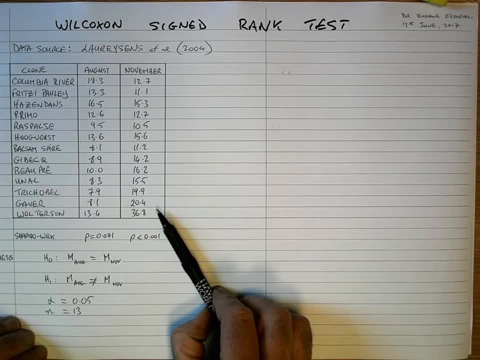 twice, in August and November, which means that these are paired data and normally, when we want to see if there's a significant difference between paired sets of data, we might use a T-group. So we're going to use a T-group and we're going to use a T-group and we're going to 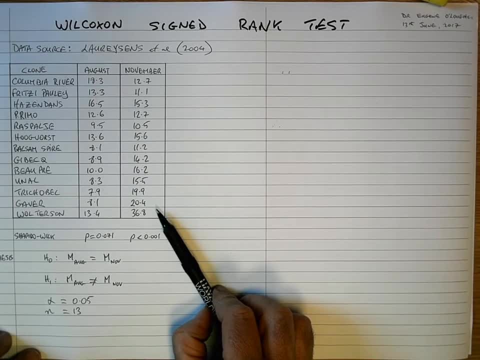 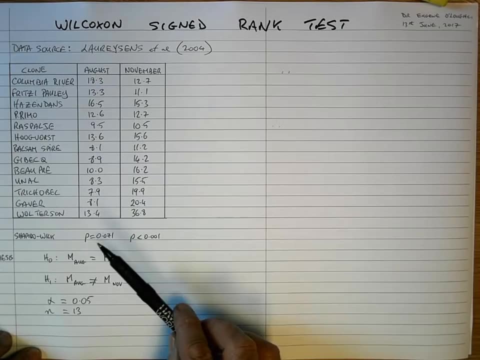 use a student T-test, but we can't use that if one or more of the samples are not normally distributed. If that's the case, then we use the Wilcoxon signed rank test. So before this video, I've conducted a quick Shapiro-Wood test on each of the August and November sets of data. 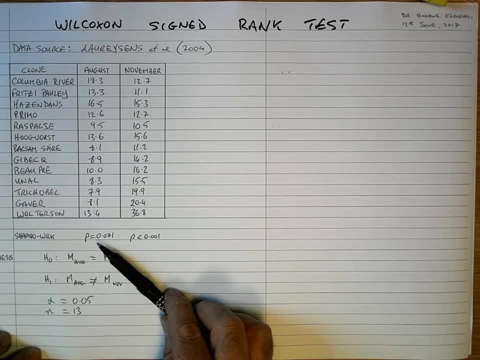 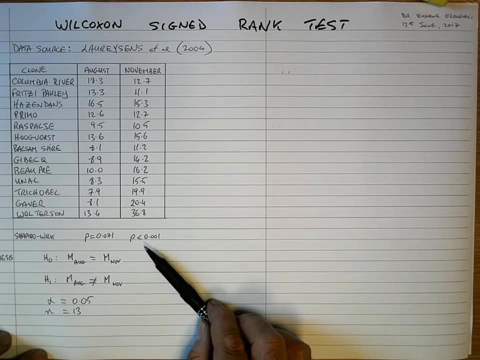 At alpha value at 0.05. I've scored a p-value in August of 0.071, which indicates that the data are normal, but the p-value is less than 0.001 for the November figure, indicating that the data are not normally distributed. And I think if you look at the data you can see that, particularly the last. 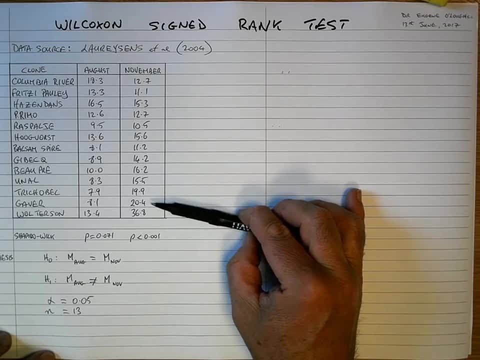 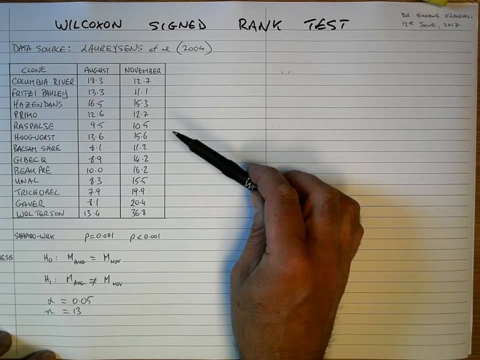 three values here are very, very high and that they are skewing the November data. therefore, it's not normal. We cannot use a T-test and we must use a non-parametric test, in this case a signed rank test. So, as always at the beginning of a statistical test, let's set out our null and 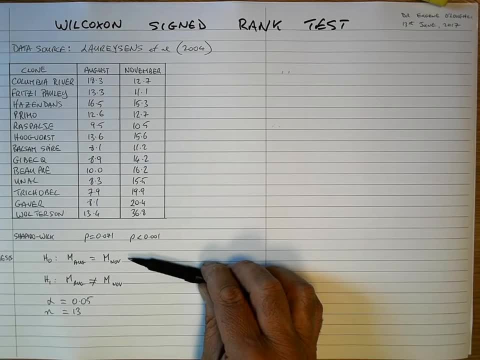 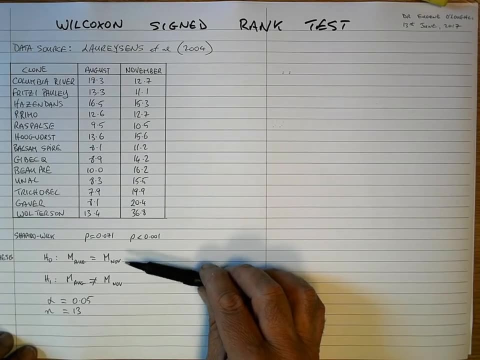 alternate hypotheses. Our null hypothesis is that the median difference between the pairs of observations is zero, and note that the hypothesis is based on the median. Our alternative hypothesis is that the median difference between pairs of observations is not zero. We're going to conduct our test if we have an alpha value of 0.05 and we've got 13 pairs of data, so we have a value of. 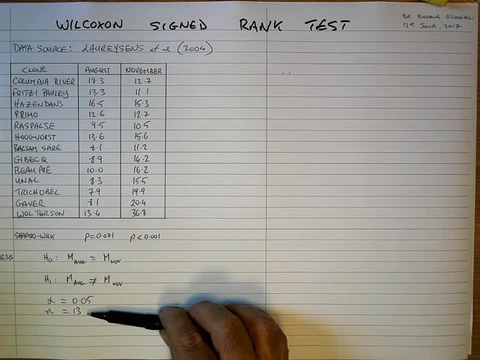 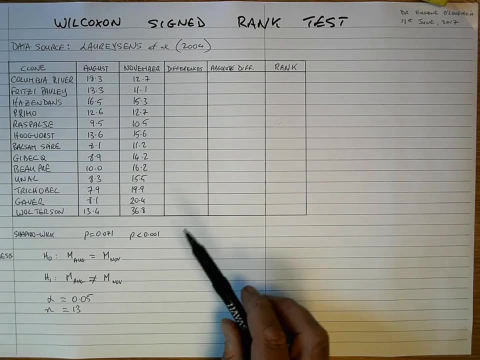 n of 13, which we are going to need a little bit later on. So to set myself up for doing the calculations, I'm just removing that top sheet and I'm using the same data and I've added in three extra columns that I'm going to need to use here to calculate the 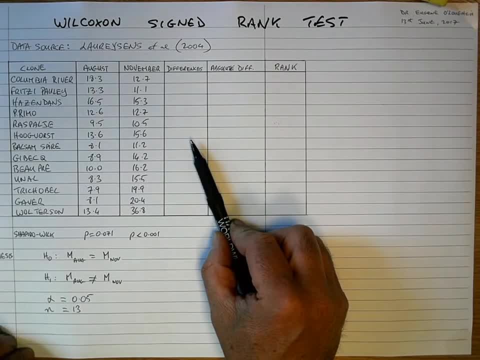 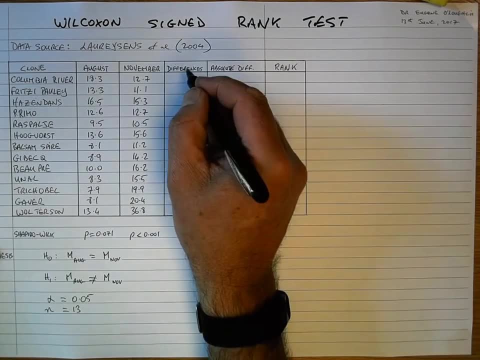 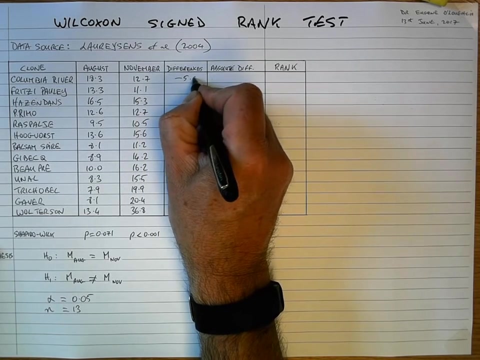 test statistic for this Wilcoxon signed rank test. So the first of these here is: I want to note the differences between the November and the August data, which is simply subtracting one value from the other. So 12.7 minus 18.3 is equal to minus 5.6.. 11.1 minus 13.3 is minus 2.2. 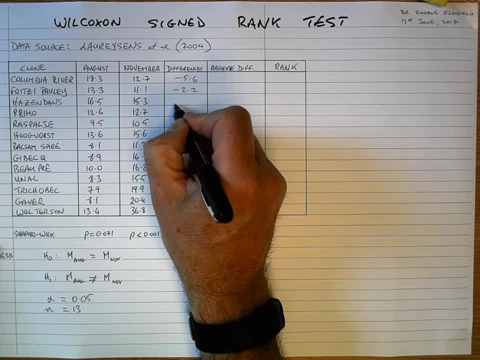 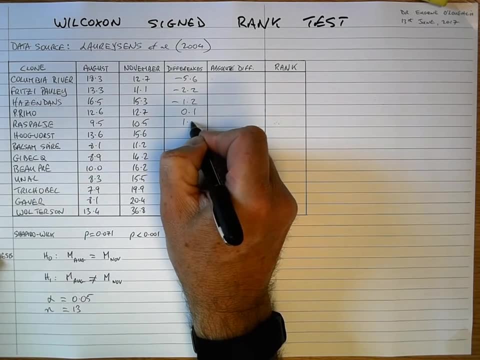 and 15.3 minus 16.5 is minus 1.2. and then the next one. I get my first positive value. There's a difference of 0.1, and then the next one is a difference of 1.0- 2.0, and I'm just going to fill. 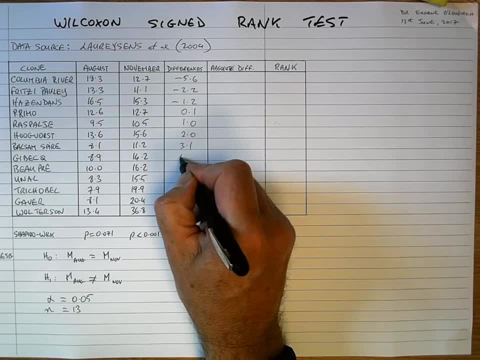 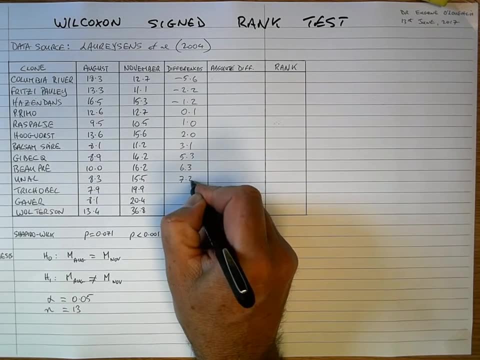 this out. I've previously calculated these values here: the differences between the November and the August data, 7.2, 12.0- and we've got some very big differences down here near the end, particularly the last one, which is the number of errors. So we're going to add in two more values and we're 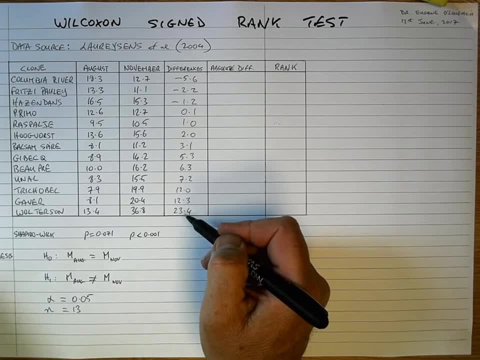 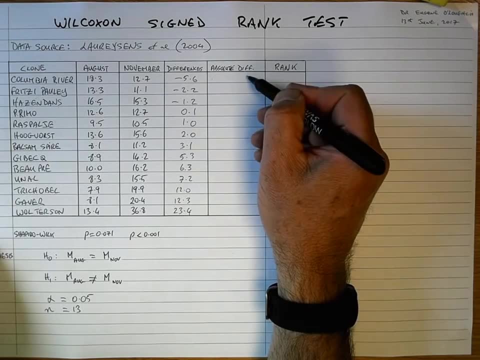 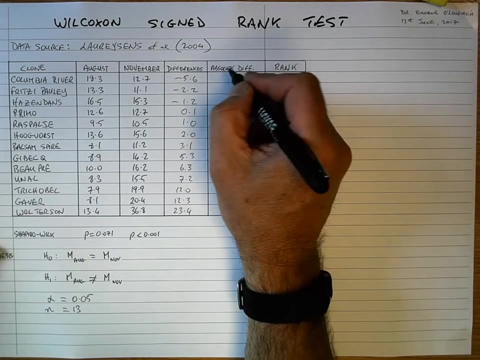 value 23.4. so a huge difference here. at the end, again emphasizing the abnormality of some of the data here and then in my next column, then I just need to take the absolute difference, which is simply removing any negative signs that you see in this column here. so the absolute value of minus. 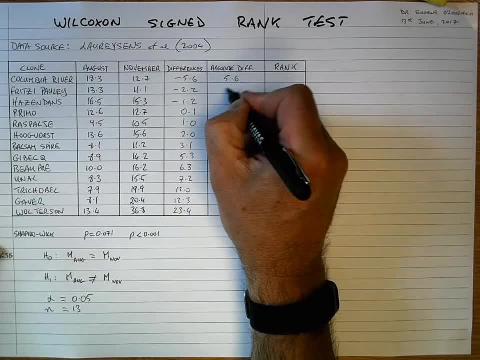 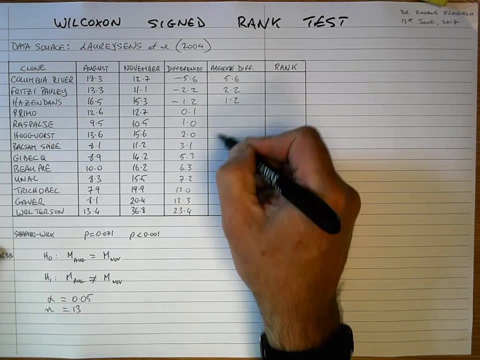 5.6 is 5.6. absolute value of minus 2.2 is 2.2. the absolute value of minus 1.2 is 1.2, and then the absolute value of all the positive values here is the same as they are as far as the. 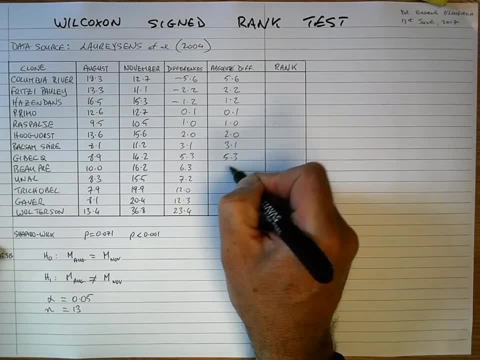 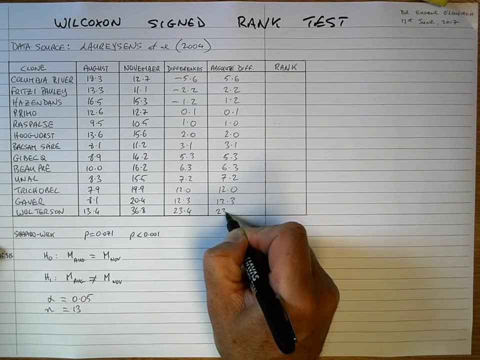 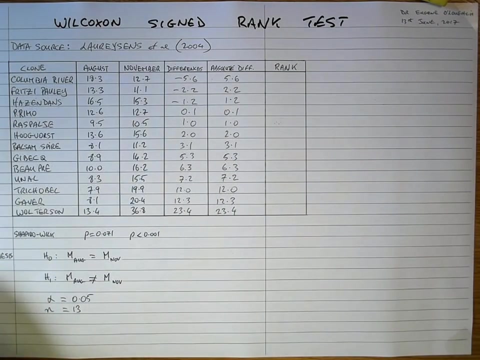 differences are concerned, so we've no minus sign here, so we're just going to write all of these out as we see them in our data. so our last absolute value is 23.4. our next job, then, is to rank these absolute values. this is why we need the absolute values, because we don't want to rank any negative. 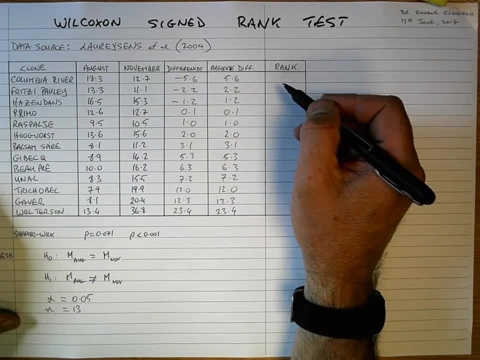 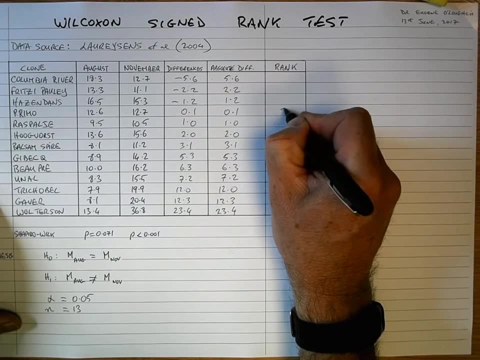 values, but we want to rank all of them and we're going to rank them from the smallest to the largest value. so, reviewing this absolute difference column here, I note that my smallest value, which gets a rank of 1, is my value of 0.1. my next smallest value is the figure here beside it: 1.0. so I'm going to write. 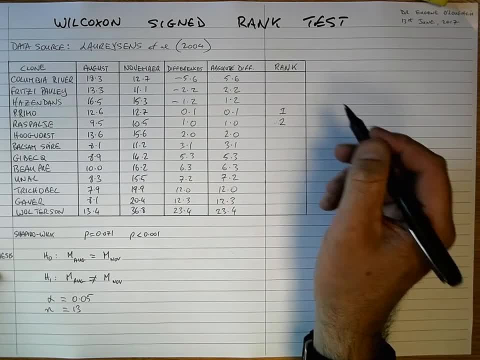 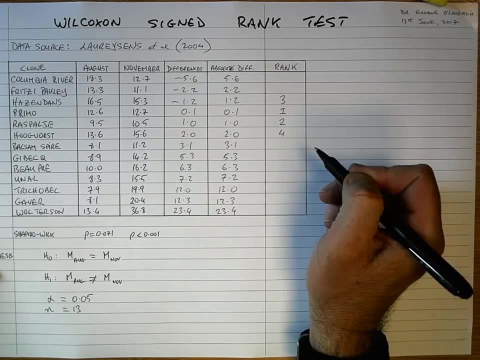 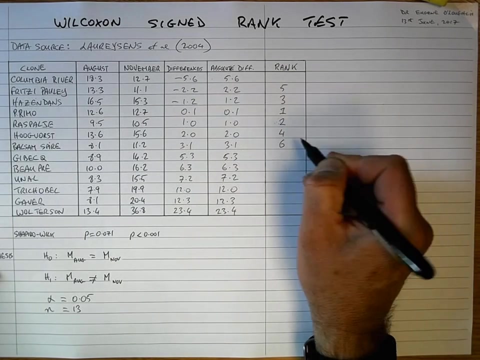 that as a rank of number 2, and my third figure is 1.2. so as they are increasing, I'm adding in the ranks. the next highest figure is 2.0, that's gets a ranking of 4. the next highest figure is 2.2, gets a ranking of 5, and then the next highest is 3.1, which gets the ranking of 6. 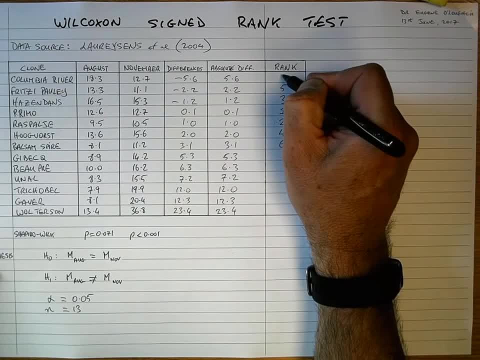 next highest is up here at the top, 5.6, and that gets the ranking of sorry, the next highest one here is 5.3, which is rank number 7, and then the next highest one is 5.6, which gets a rank of. 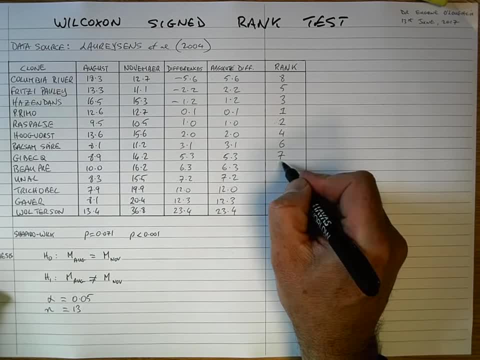 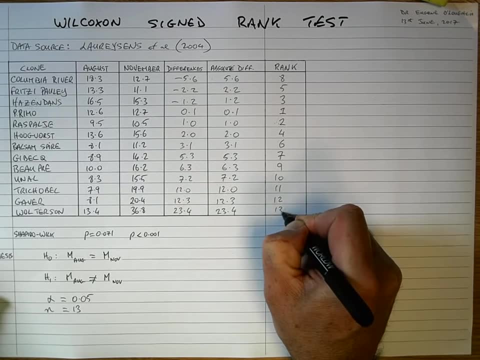 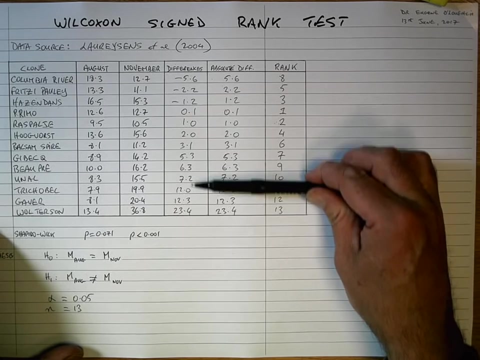 number 8. the next highest one then is ranking of 6.3, which is a ranking of 9, and then you can see these are all sequential here at the end. so the last sets of rankings are easy to determine here. so our just to recap here for a second: we our differences. we are very, very important that we. 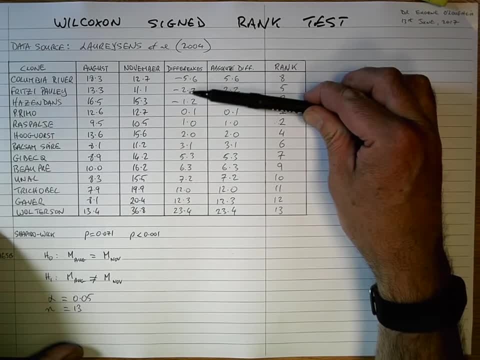 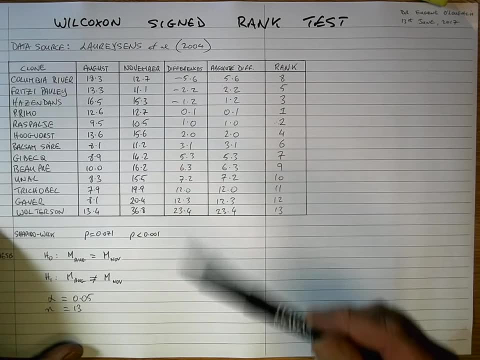 know the sign, because this is a Wilcoxon signed rank test. so we need to know all the positives and we need to know all the negative differences, and then we need to know the ranks of all the positives and the ranks of all the negatives so that we can sum them. so we need to know the rank. 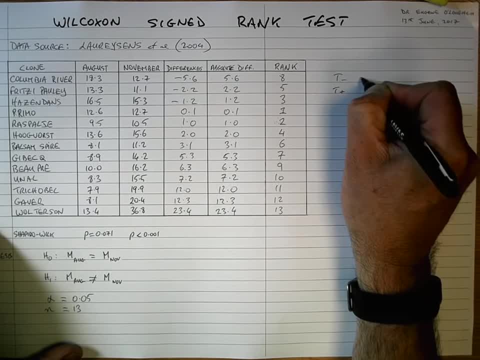 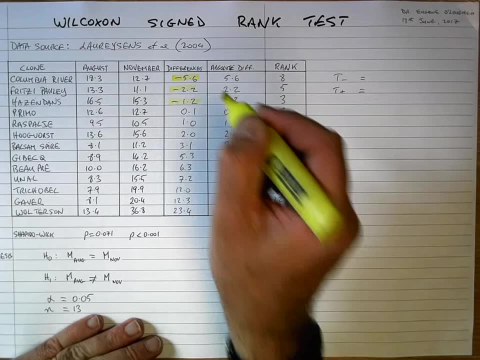 sum for the t pluses and for the t minuses. so to do that I'm just going to use a highlighter here, so I need to highlight all of the negative values, or conveniently here at the top, and then select the ranks for each of those there. so 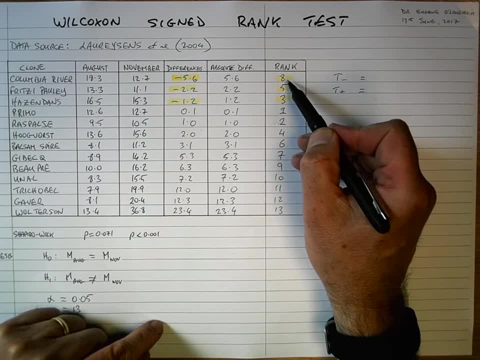 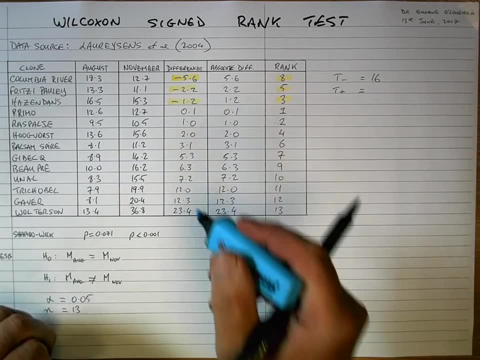 all the negative values. so the rank sum of the negative ranks here is 8 plus 5 plus 3, which is 16, and then I'm going to do the same for all the positive values. so they're all conveniently here for me. so these are all the positive differences and these are all the positive ranks. this is going. 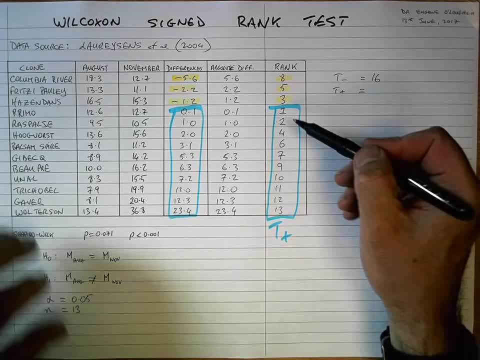 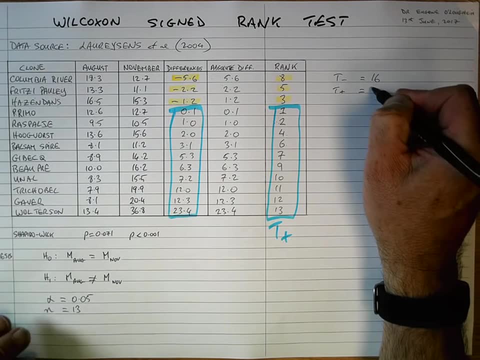 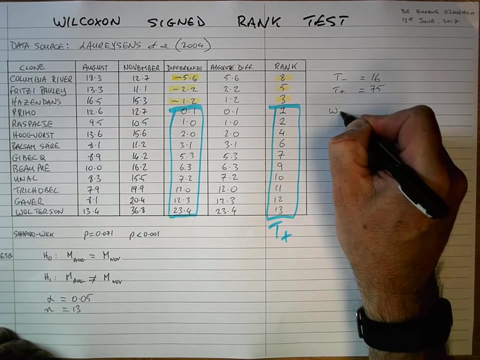 to give me my t plus all the positive ranks. so when I sum up all these values here- one, two, four plus six plus seven and so on, I'm going to get a t value here, t plus value of 75. the Wilcoxon ranked assigned rank test statistic is called w, so my w stat what's the test statistic? 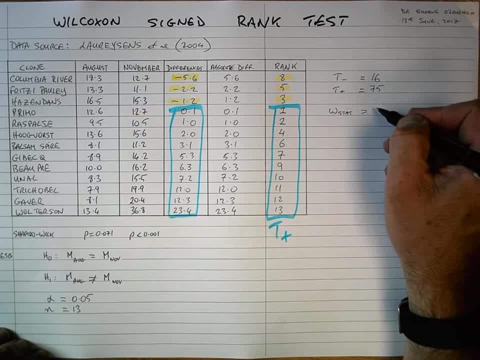 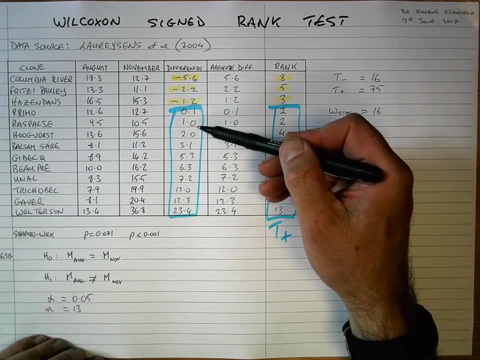 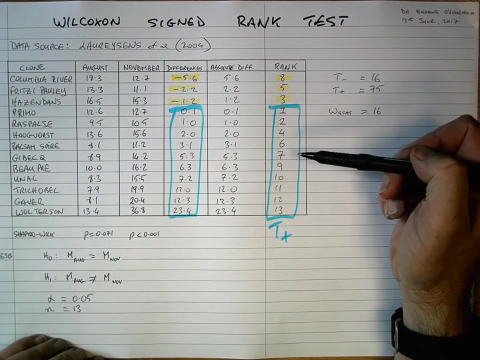 well, it is the smaller of these two values here. so the w stat is 16.. just to check back for a second: if any ranks are the same, so if you get two different absolute differences which are the same, you take an average of the ranks for those two or three ranks in that case. so now our test statistic. 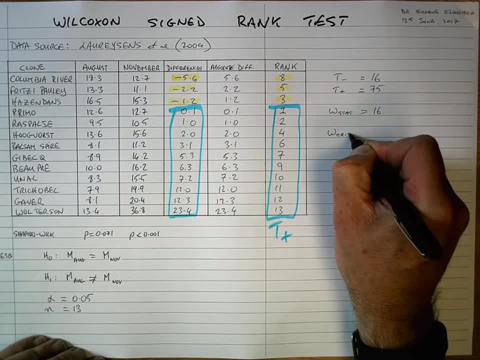 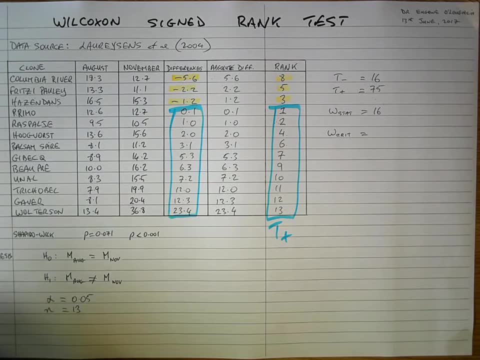 has a value of 16.. we now need to determine a critical value so that we can compare our test statistic with a critical value to determine if there is a significant difference. so to do that, I'm going to use a critical values of the Wilcoxon. 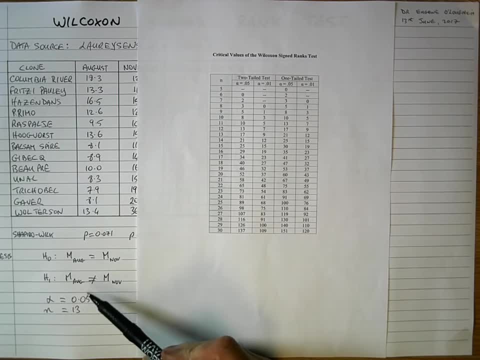 signed ranked test table. and to check back here: right back at the beginning in the video I stated that our alpha value was 0.05, that N was 13 and you can also see that we are doing a two-tail test here. no direction is specified, so it is a two-tail test. so from my table, the first column gives me: 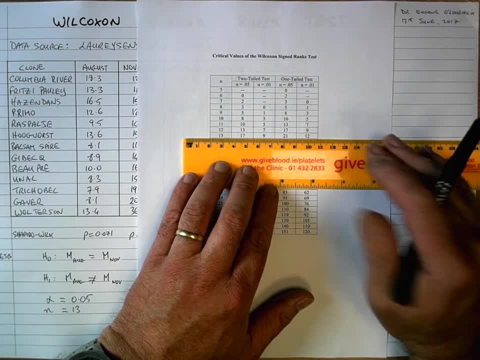 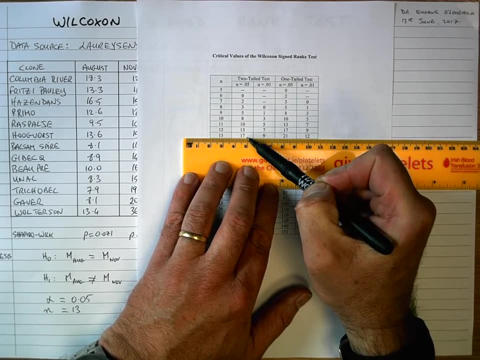 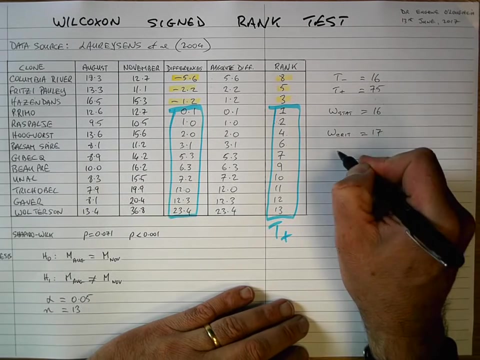 the row I need to use. so n is equal 13, a two-tailed test and alpha value of 0.05. so go down along here and we get a critical value of 17 in this case. so let me note that my w crit is 17. so in this case, here my test statistic. 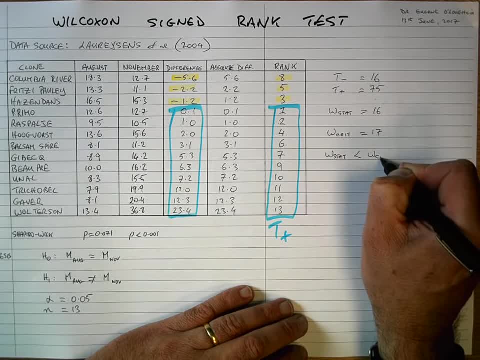 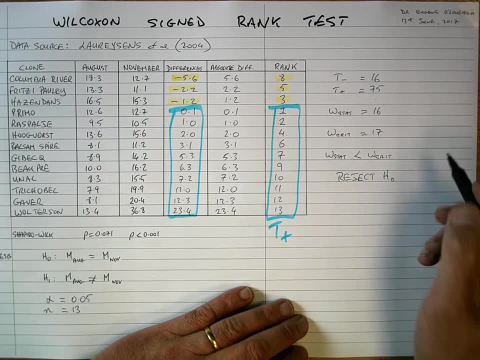 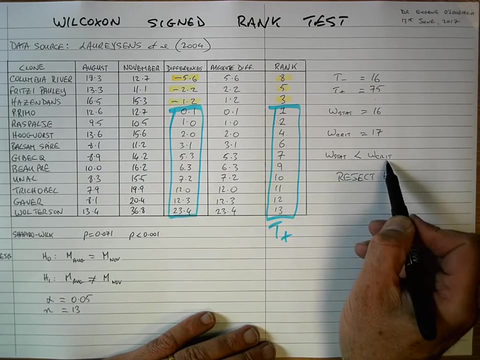 is less than my critical value and that results in here of that we reject the null hypothesis, we reject h0 and be very, very careful with this because many statistical tests if you- it is you- only reject when the test statistic is greater than the critical value. but in the wilcoxon signed 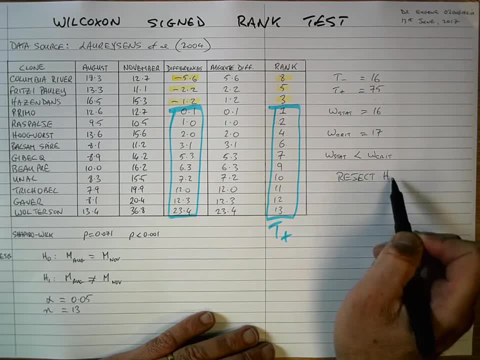 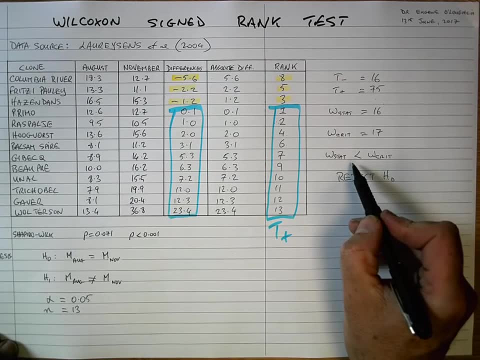 rank test is the reverse of that. so we're looking for: if we want to reject the h0, we have to get a test statistic less than the critical value. so here 16 is less than 17. therefore our w stat is less than w crit. we reject h0. so in other words, we are rejecting this statement over here that. 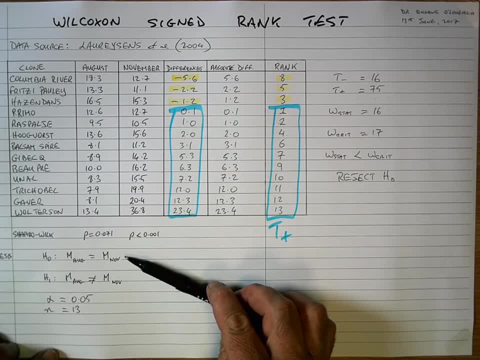 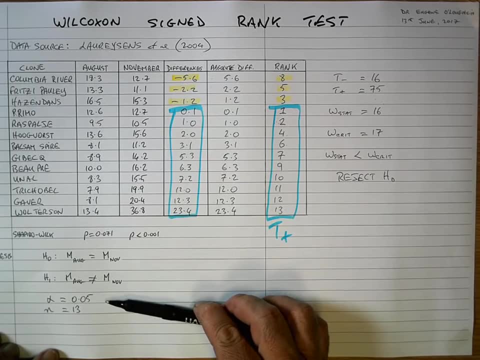 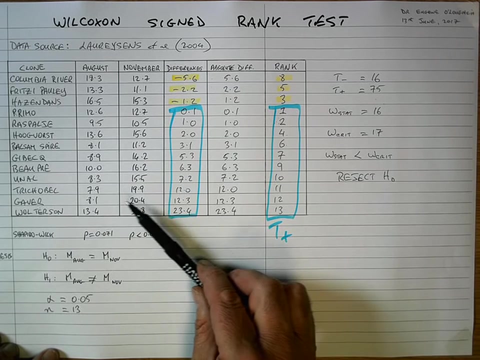 the median differences between all august and november are zero, so we are rejecting that in favor of the alternative hypothesis that the median differences are not zero, and we're doing all this at an alpha value of significance of 0.05. so, in conclusion, then, we have found a significant difference between the concentrations. 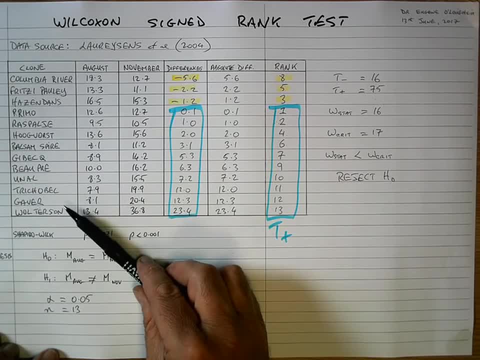 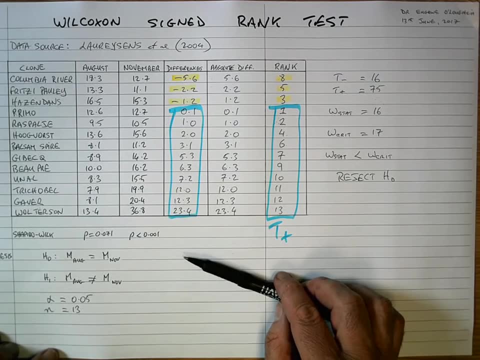 of aluminium between the august and november data for the popular tree clones. so that's how you perform a wilcoxon signed rank test by hand. i hope you found this video useful. thank you for your attention you.